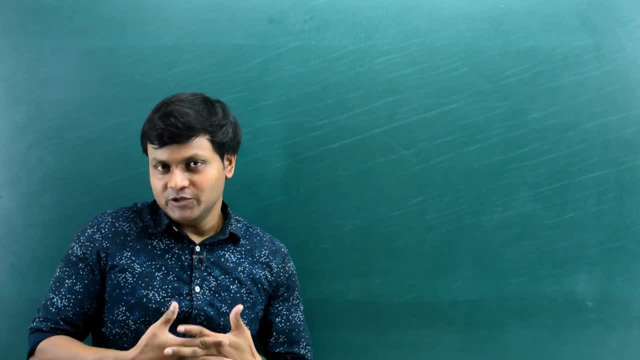 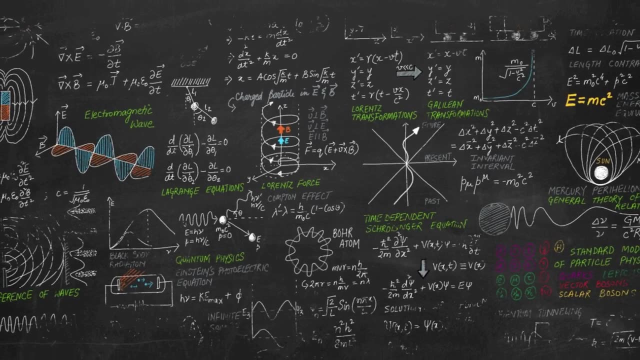 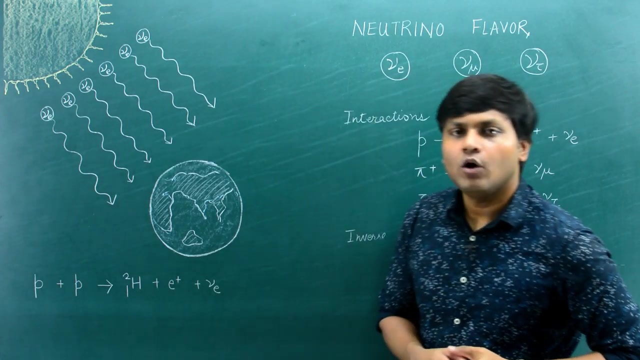 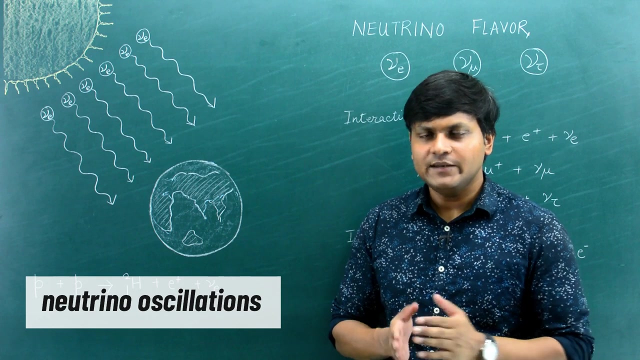 I'm joking, so this is what this video is going to be all about. welcome to my channel. so, before we talk about this multiple personality of neutrinos or, to be more precise, neutrino oscillations, let me give you a context to this whole thing. you see, at the core of our Sun, 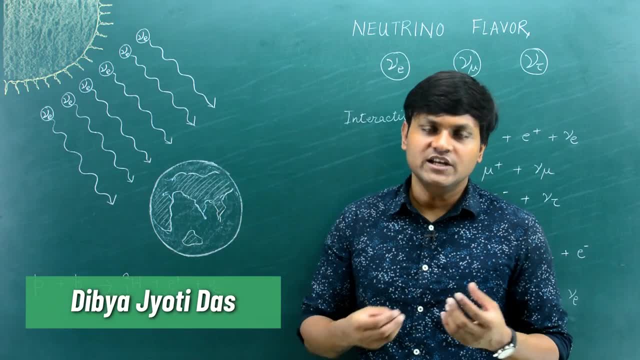 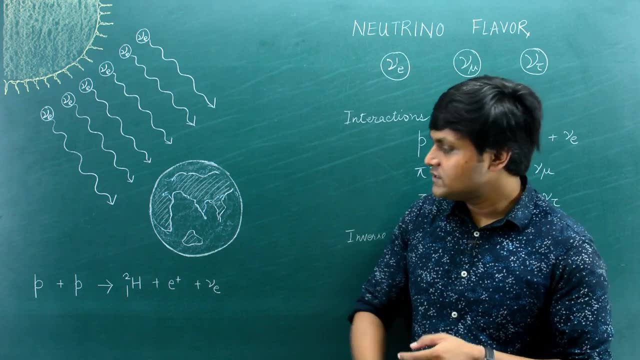 thermonuclear fusion reactions are happening all the time, which leads to the creation of huge amounts of energy and large number of neutrinos. one of the reactions that happen at the core of the Sun is two protons. they come and fuse together on the very high temperature and pressure leads to the creation of a deuterium nuclei. now, a deuterium nuclei consists of one proton and one neutron, so that means in this process two protons. they not only fuse together, but also a beta decay happens, where a proton gets converted to one neutron, which is the beta decay process. 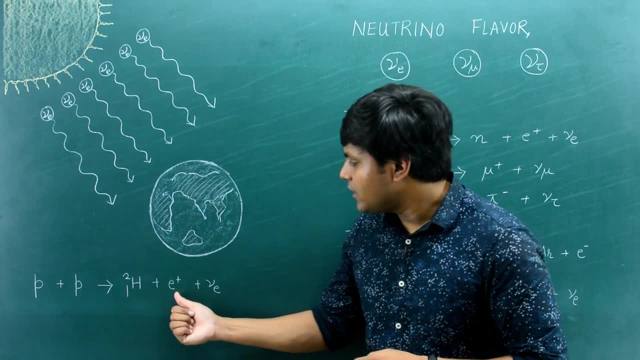 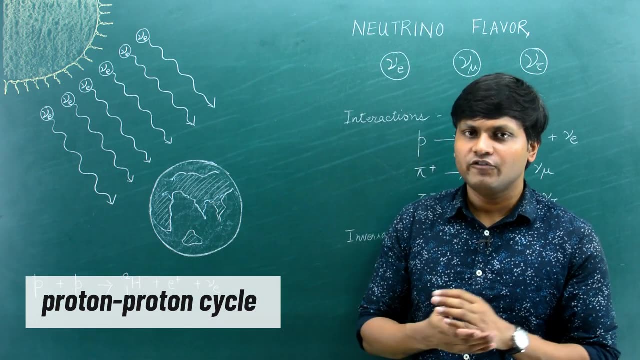 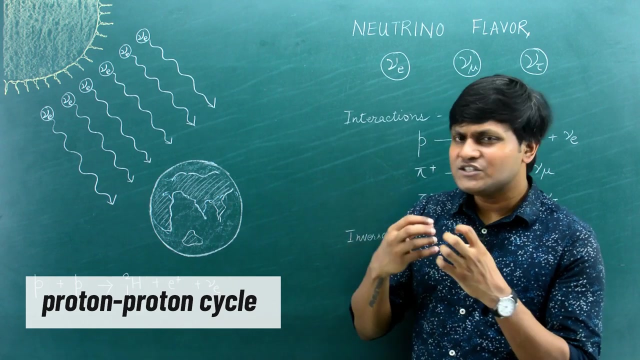 gets converted to a neutron, therefore leading to the emission of a positron and a neutrino. so this is part of a broader proton proton cycle of reactions, which is one of the dominant cycles of nuclear fusion reactions that happen at the core of our sun. therefore, vast majority of the 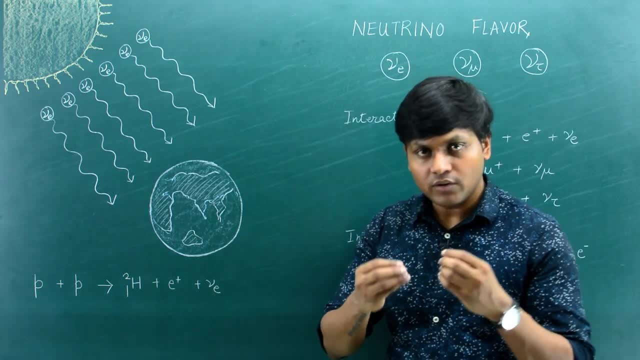 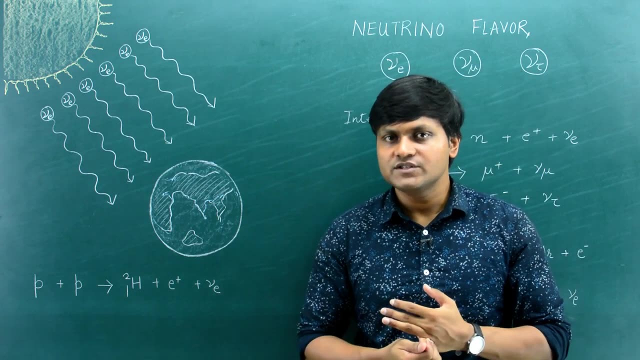 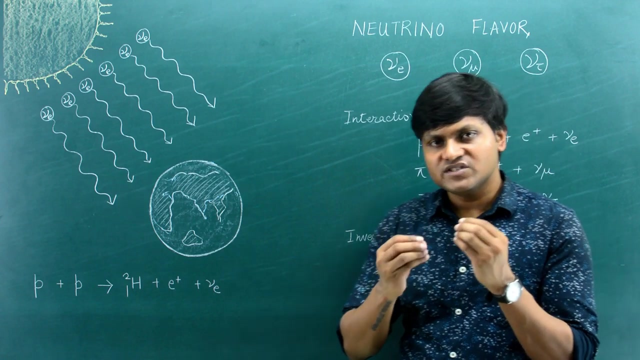 neutrinos which are emitted from the sun are essentially electron neutrinos. now, when scientists develop the technology to actually detect these kind of neutrinos, they tried to find out the flux of these neutrinos coming from the sun and they found a very interesting puzzle. so it turns: 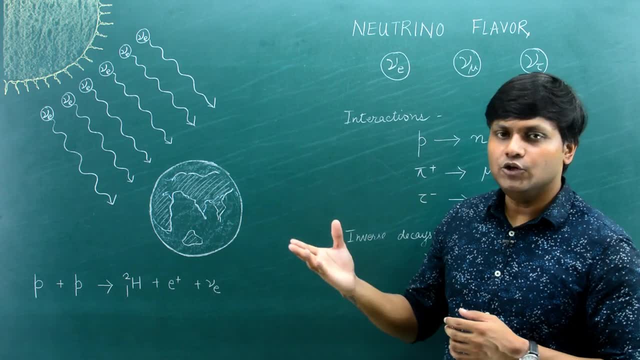 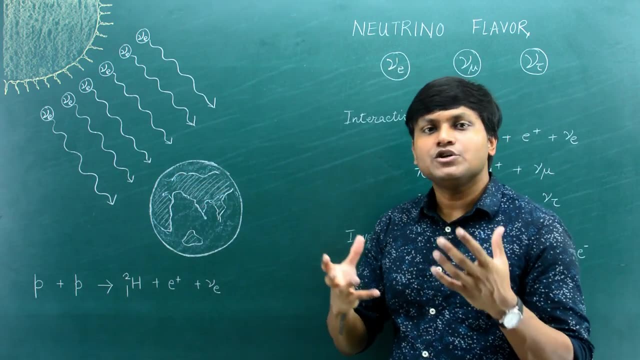 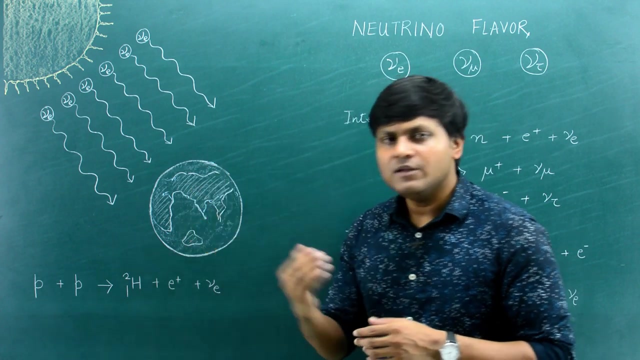 out that the theoretically predicted value of the electron neutrinos that are supposed to come from the sun to the surface of the earth and the experimentally measured flux of neutrinos on the surface of the earth were not matching. in fact, the experimentally measured flux of neutrinos was much less, almost one-third to two-third. 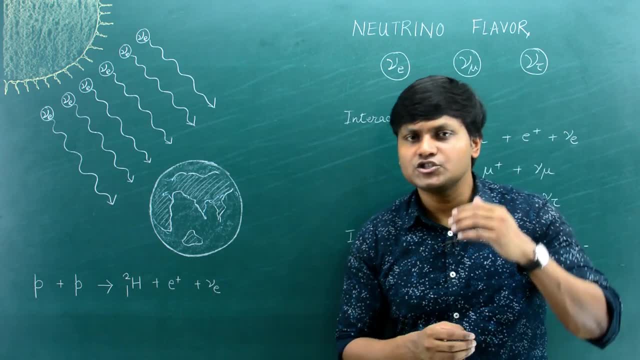 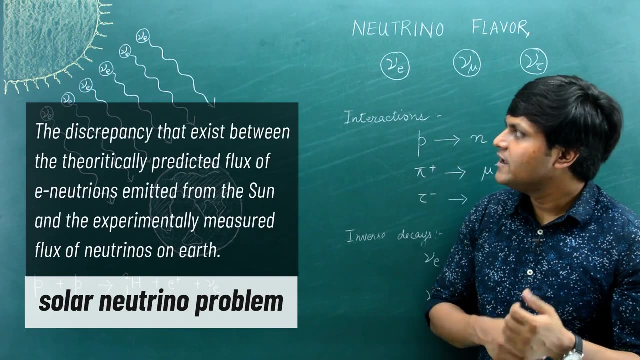 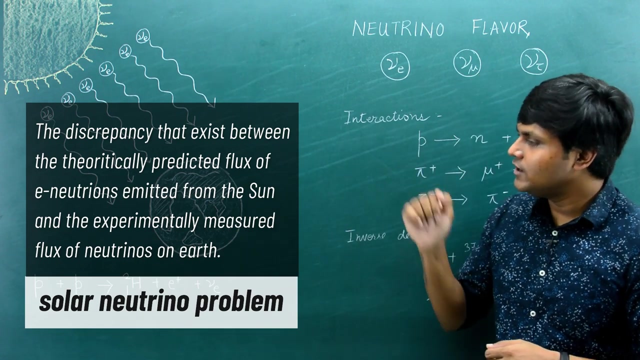 compared to the theoretically predicted value. this is known as the solar neutrino problem or the solar neutrino deficit. it simply refers to the discrepancy that exists between the theoretically predicted flux of the electron neutrinos emitted from the sun and experimentally measured flux of the neutrinos on the surface of the earth. so this is something that puzzled scientists, for. 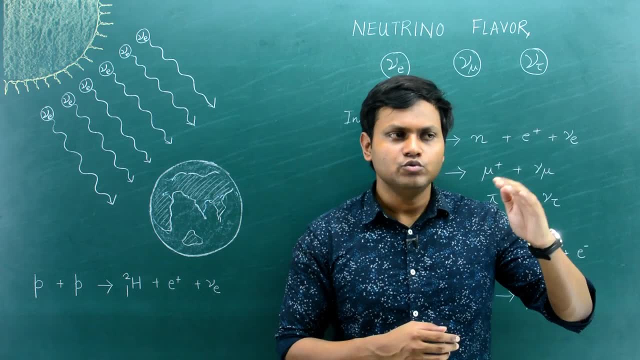 a very long time. so let's take a look at the experimentally measured flux of the electron neutrinos on the surface of the earth. so this is something that puzzled scientists for a very long time, from the 1960s to the very beginning of this century, before it was resolved, and it was a big. 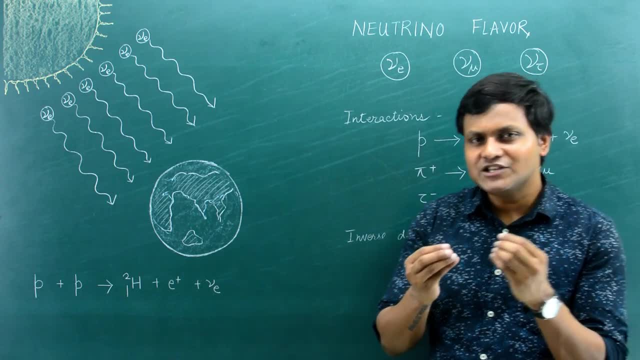 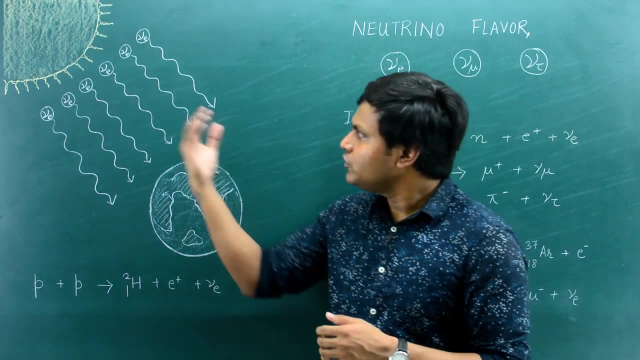 challenge to come up with a kind of an explanation of why this kind of a discrepancy was happening in the first place. now you need to understand that the neutrinos which are coming from the sun were essentially electron neutrinos. now, what is an electron neutrino? see, you see, there are three. kinds of neutrinos. one is the electron neutrino, the muon neutrino and the electron neutrinos are, and the tau neutrino, which is also known as the flavor of neutrinos. they belong to the electron family, the muon family and the tau family respectively. now, these are very much distinct. 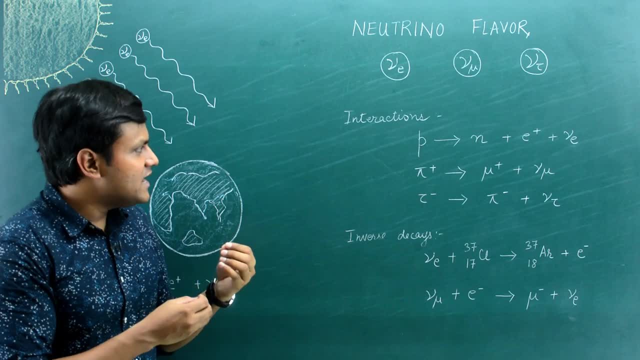 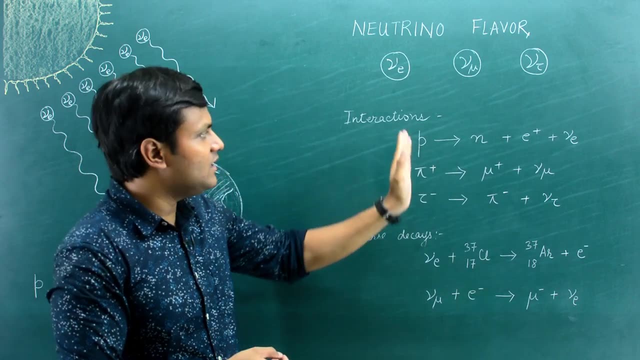 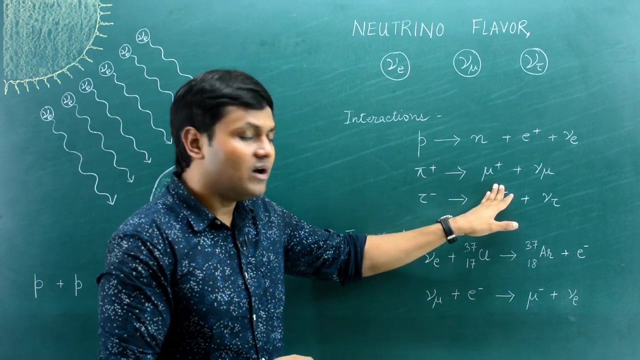 neutrinos. now why do i call them distinct? this is because they are the result of different kinds of interactions. so, for example, when a proton decays to become a neutron, you end up getting an electron neutrino in the process. when a anti-pymeson decays into a electron neutrino, you end up getting an. 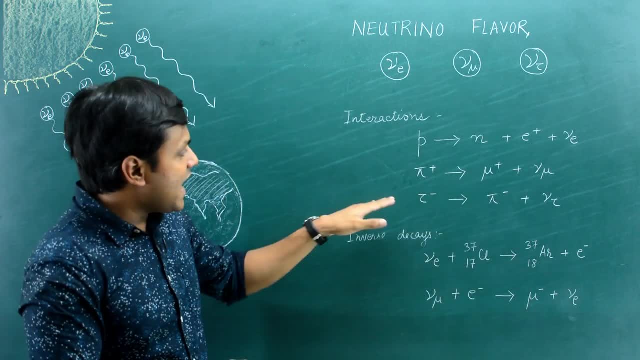 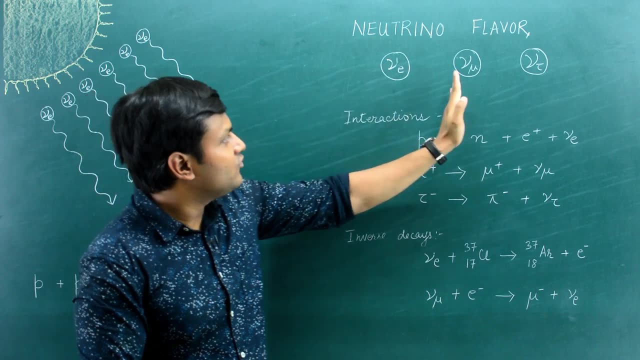 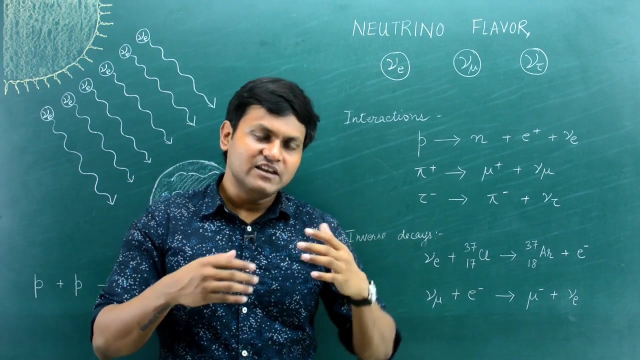 anti-muon, you end up getting a muon neutrino. and when a tau particle decays into a pymeson particle, you end up getting a tau neutrino. so these three distinct neutrinos, the electron, muon and the tau neutrinos, are the result of different kinds of interactions. in fact, the interactions that these 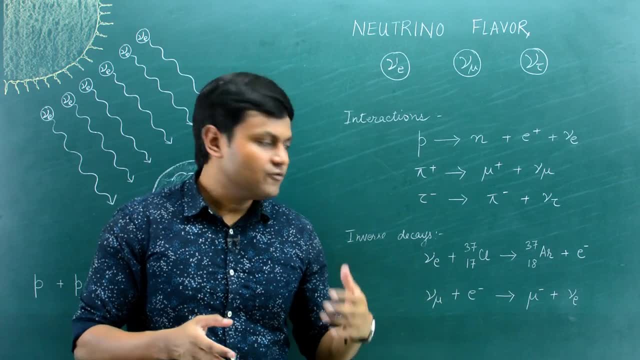 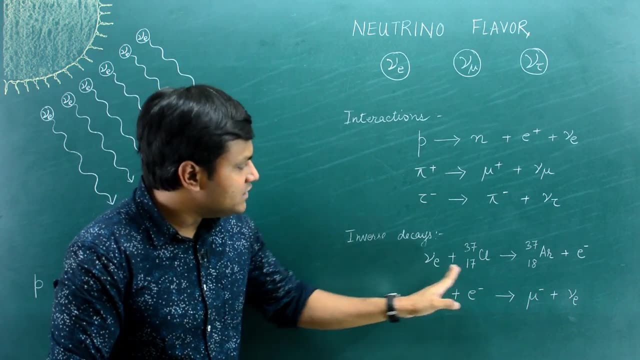 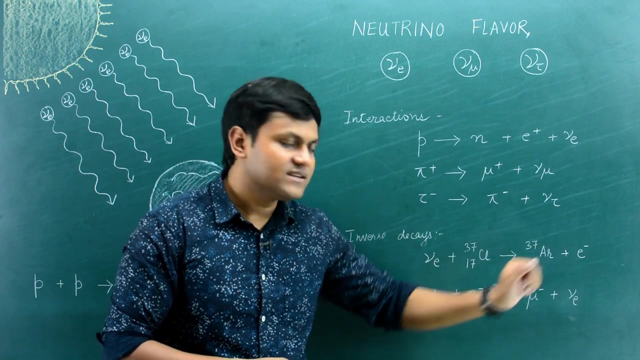 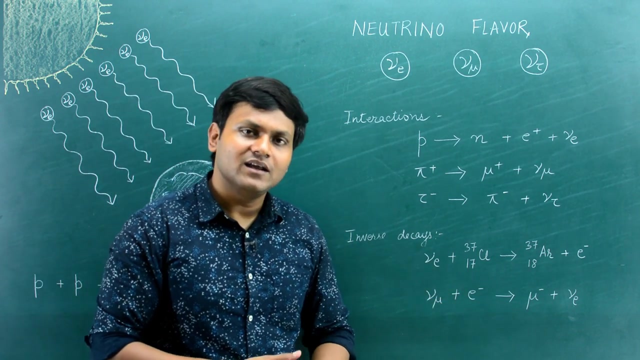 particles can induce are very much distinct from one another. so, for example, if you look at the inverse decay processes associated with these particles. so, for example, an electron neutrino can create a muon particle and an electron neutrino in the process. now you cannot interchange an. 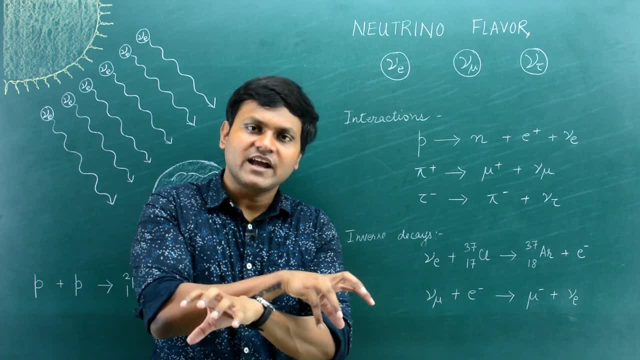 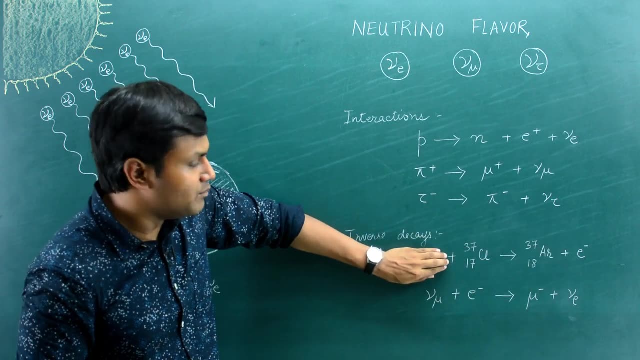 electron neutrino and a muon neutrino in two different interactions and expect the interactions to happen in the first place. it's not possible. so this kind of an interaction cannot be induced by, let's say, a muon neutrino, while the second interaction cannot be induced by a muon neutrino. 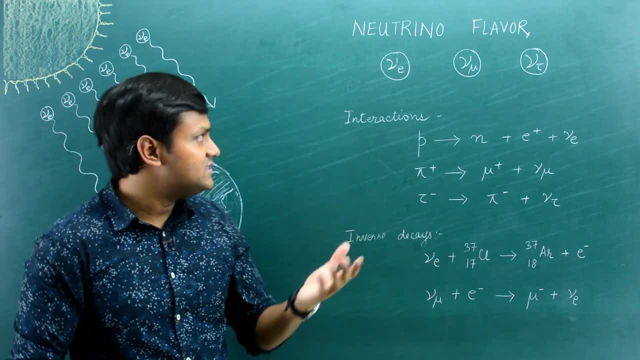 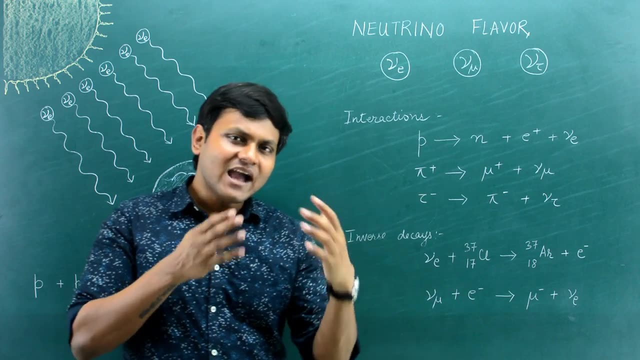 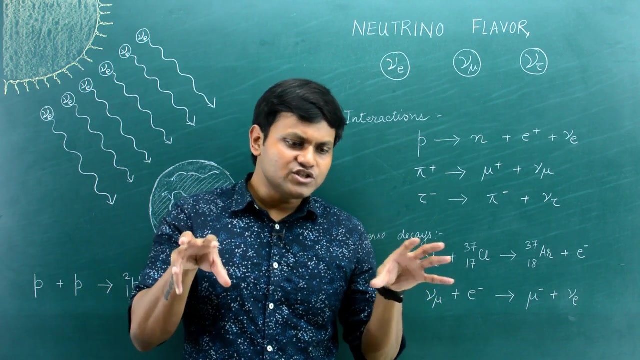 by an electron neutrino. so what i'm trying to say here is that these are in fact very much distinct particles with their distinct identities, and the reactions that they induce and the interactions from which they are released are very much distinct from one another, and you cannot just 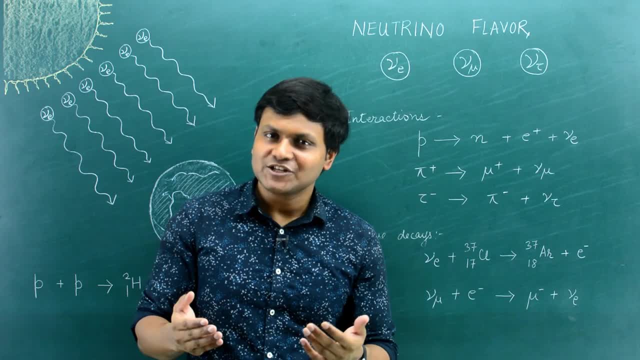 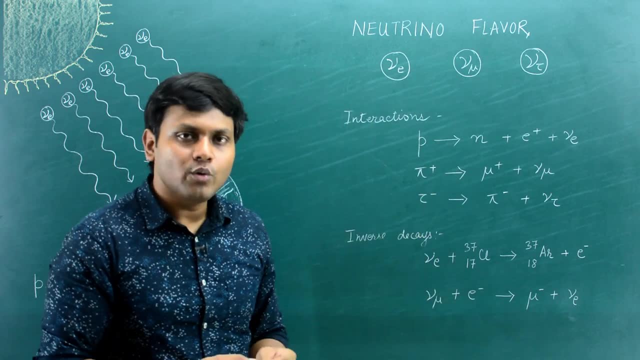 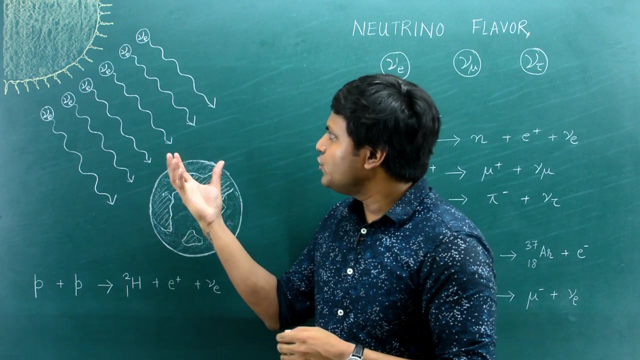 interchange one neutrino with the other and expect the interaction to happen in the first place. so that means these are very much distinct identities of three different kinds of neutrinos, which is also known as the flavor of neutrinos. so, having said that, the detectors on earth which were measuring these electron 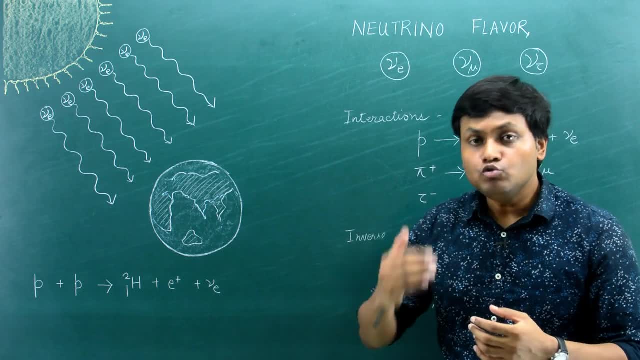 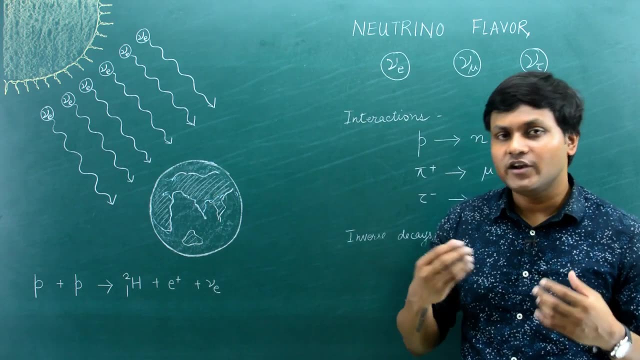 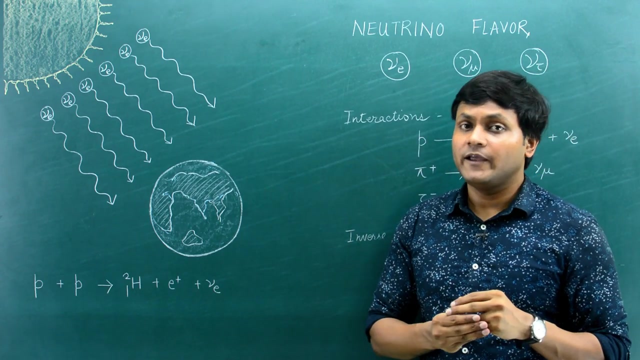 neutrinos were distinctively made to measure electron neutrinos only, and they were measuring these electron neutrinos to be much lower than what was theoretically predicted. now, one explanation for this kind of a solar neutrino deficit problem was provided by bruno ponte corvo. 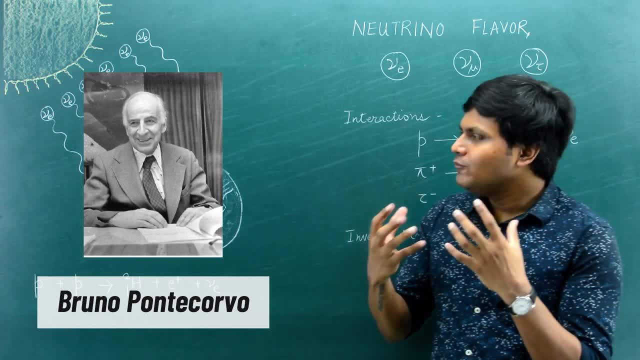 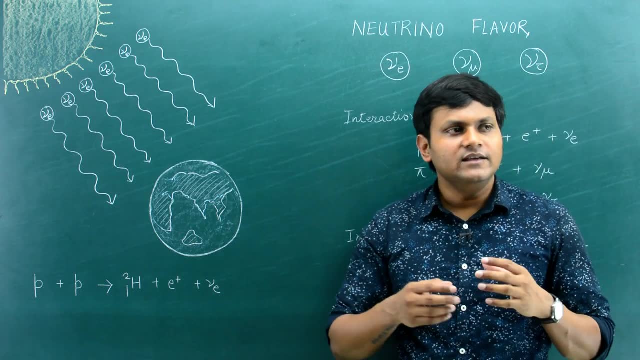 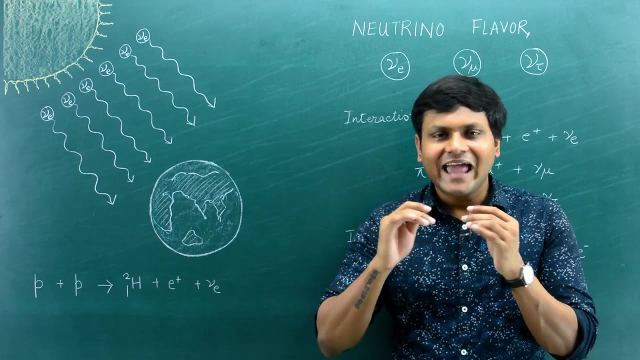 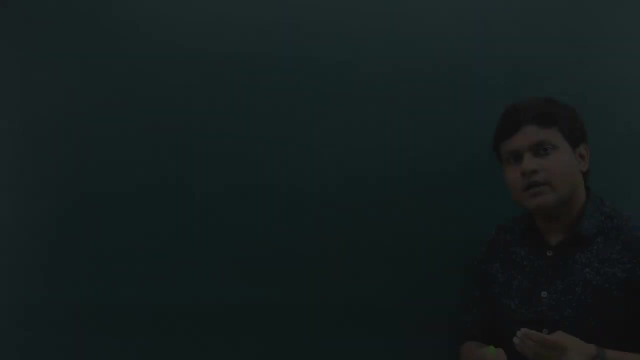 who said that there is one way we can explain this kind of a discrepancy, which is by assuming that these neutrinos are in fact the mixture of certain quantum states. and as these neutrinos travel through space, their identities transform. now, what does that mean? now you must have studied quantum mechanics right in quantum. 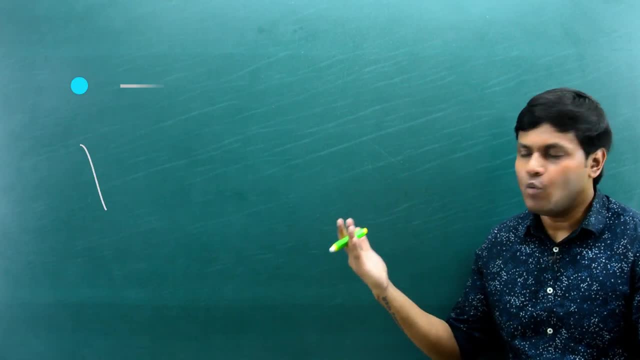 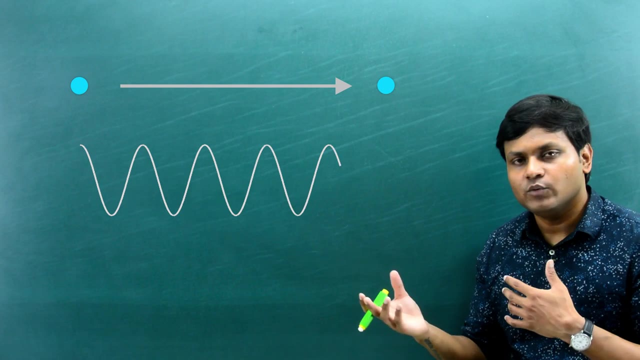 mechanics what happens. the motion of a particle as it goes from one point to another can be represented by the motion of a particle as it goes from one point to another. can be represented by the motion of a quantum mechanical wave right whose wavelength would give us an idea about 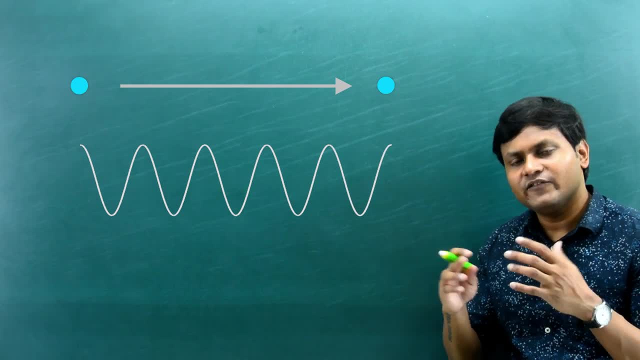 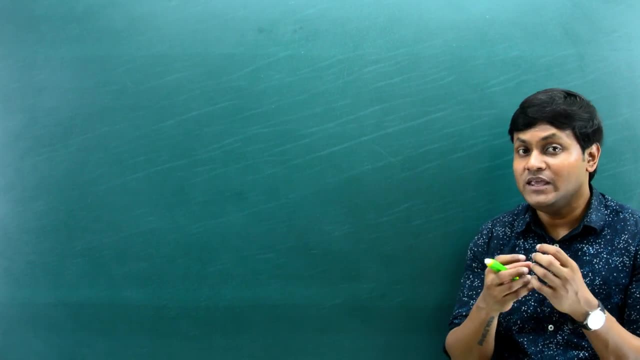 the momentum of the particle, and so on and so forth. so this kind of an idea is quite common in quantum mechanics. so when you think of the neutrino, think of the neutrino as also being an wave, but instead of it being represented as one wave, think of it as being represented by. 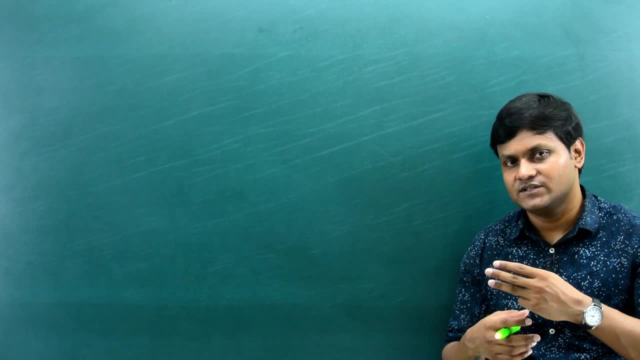 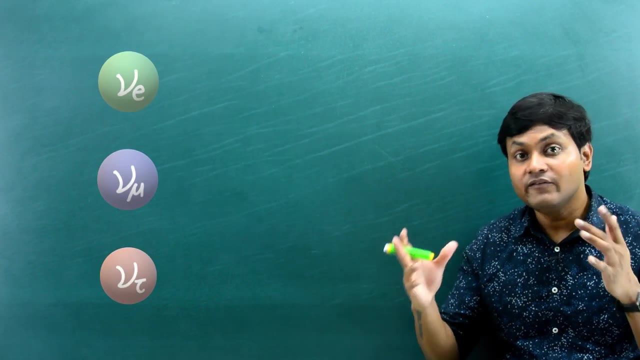 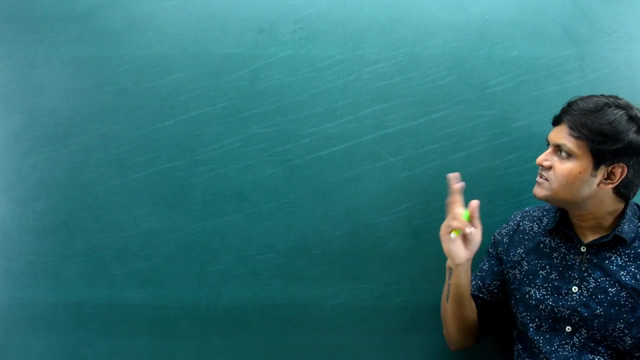 the interference caused by three distinct waves. all right, so you have the uh electron neutrino, the neon neutrino and the tau neutrino, which are the flavor states of neutrinos. they are essentially the result of the interference caused by three distinct waves, which are known as the mass eigen. 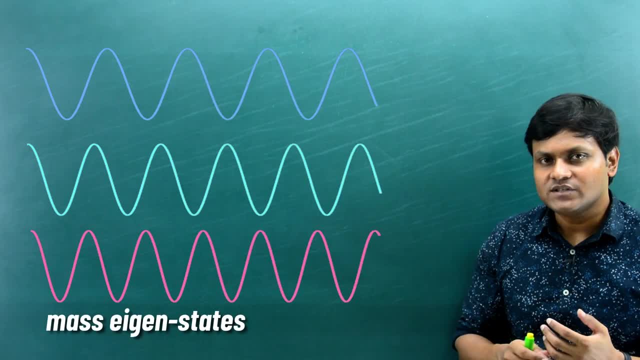 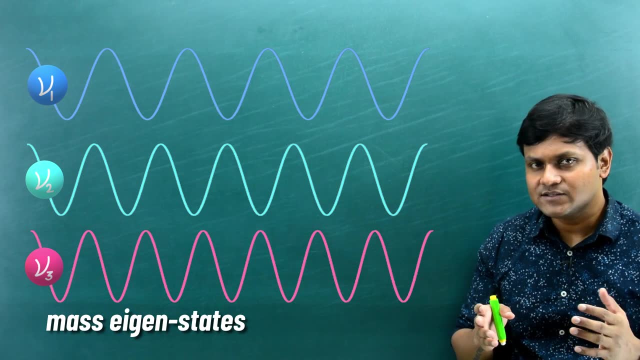 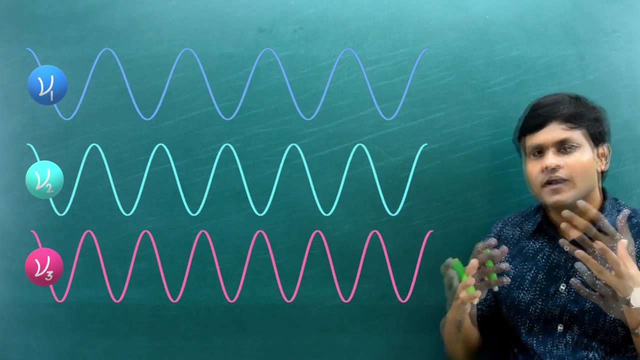 states. so these states, or these waveforms, are named as neutrino 1, neutrino 2 and neutrino 3. they are also known as mass eigen states, or i will refer to them as simply waveforms or quantum states. so what i'm essentially saying is that, or what ponte corvo essentially said is that the flavor of the neutrino is the 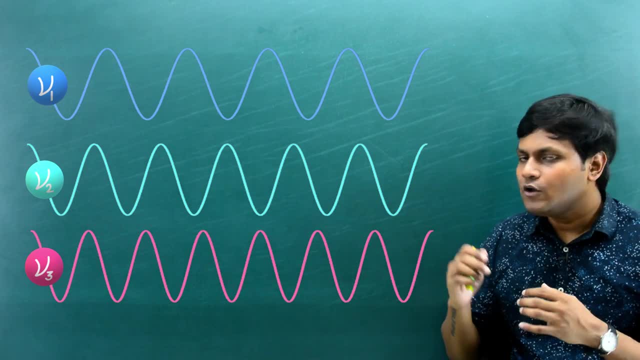 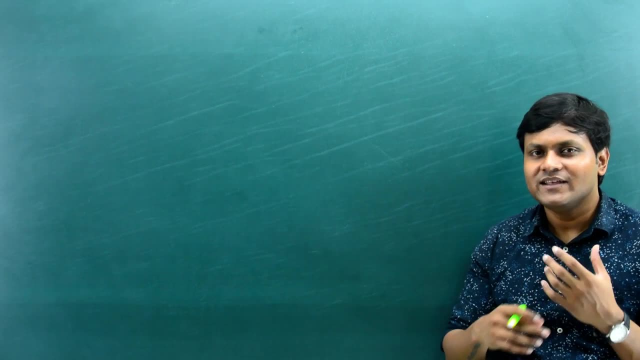 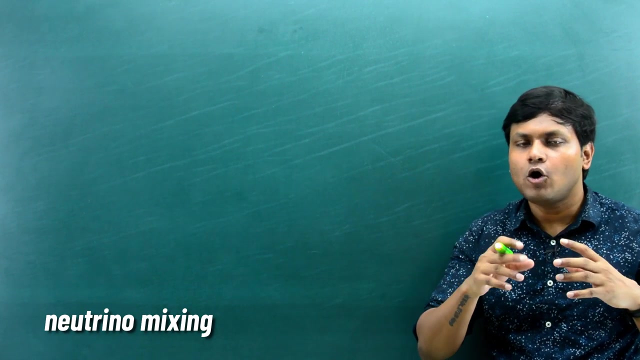 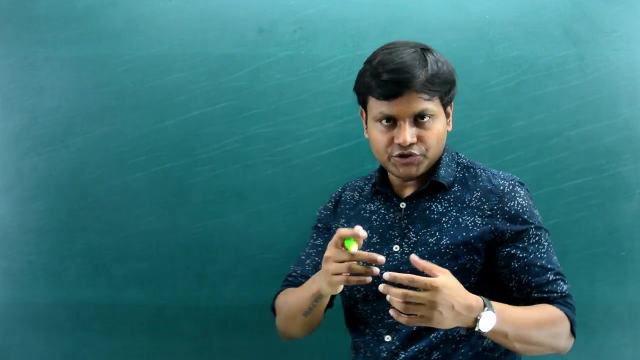 resultant of the mixing or interference of these distinct waveforms or quantum states. so that's why this is also sometimes known as neutrino mixing. so essentially, the flavor of a neutrino is the result of an interference or the mixing of the mass eigen states in certain proportions. so i can write it in this particular equation: 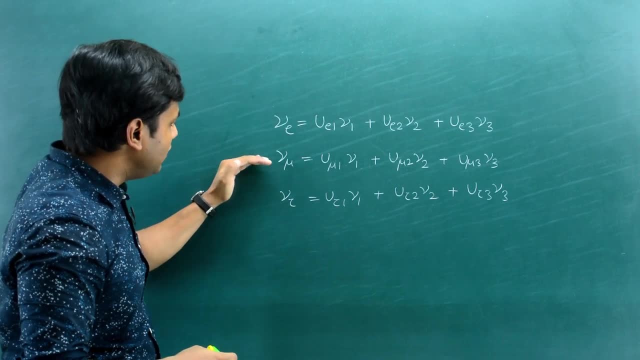 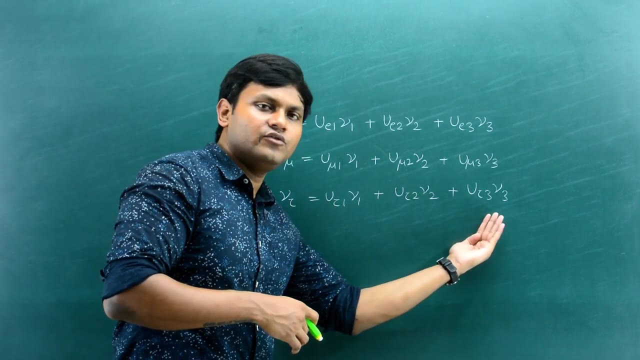 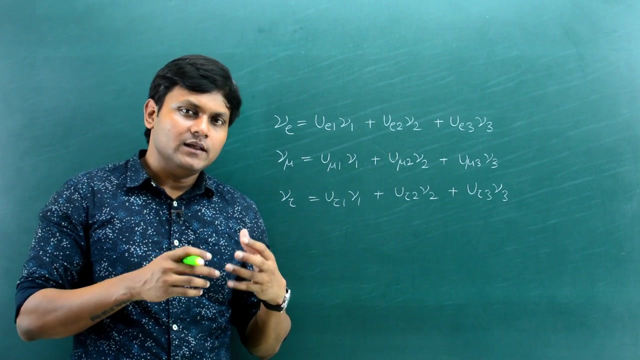 the flavor of the neutrino, the electron neutrino, muon neutrino and the tau neutrino is a result of the mixing of the quantum states neutrino one, two and three in different proportions. now we can visualize this kind of an idea using a little bit of a graphical method. 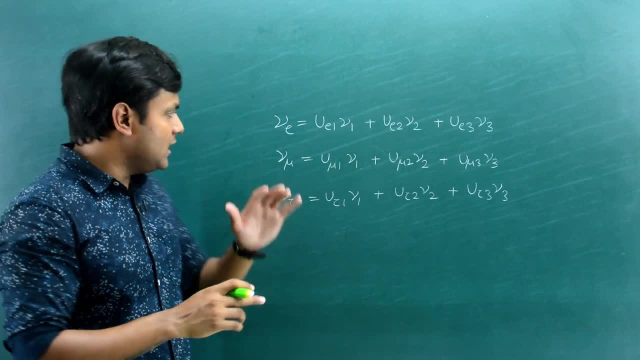 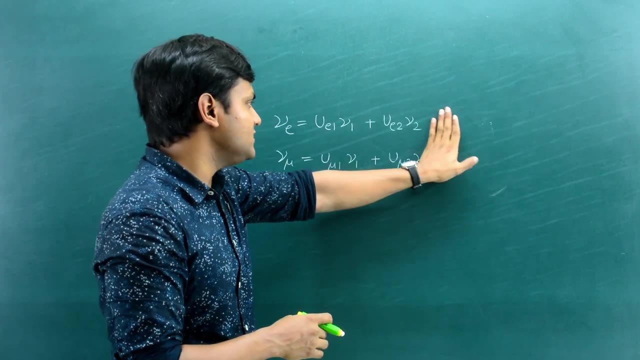 to do that, let's first suppose that we are only dealing with, let's suppose, two flavors of neutrinos and two mass eigen states. all right, so let's suppose there is an electron neutrino and a muon neutrino which are the result of a mixing. 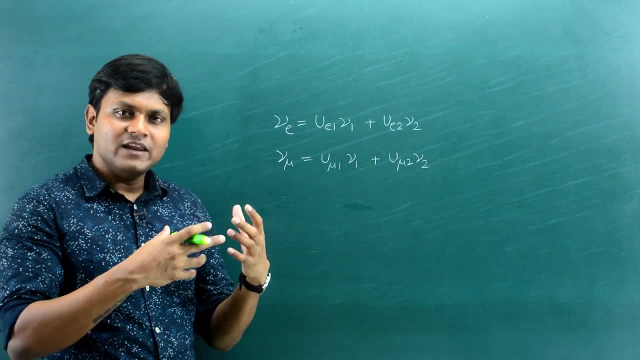 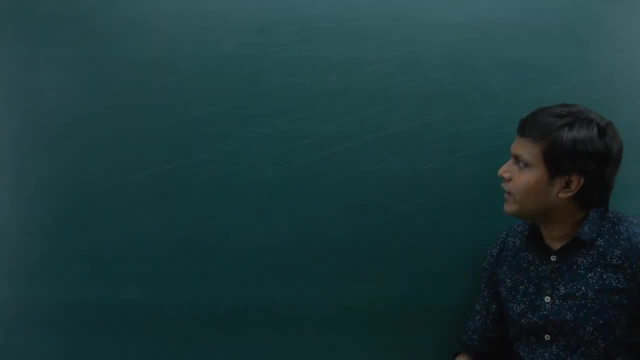 of neutrino 1 and neutrino 2, and let's see if we can visualize that and get some sense out of it, and then we will proceed to the general case later on. okay, so here we have, let's suppose, these two quantum states represented as waveforms. 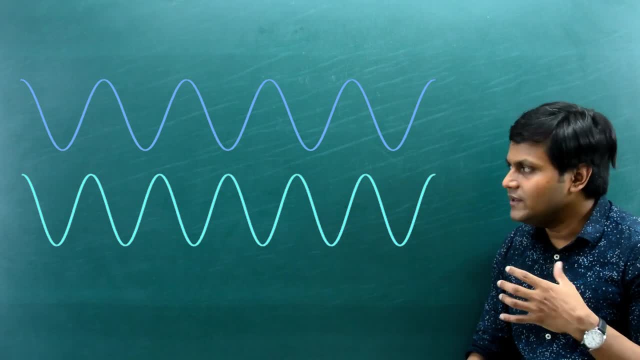 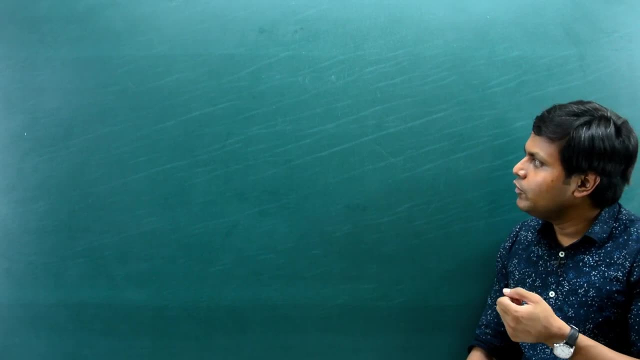 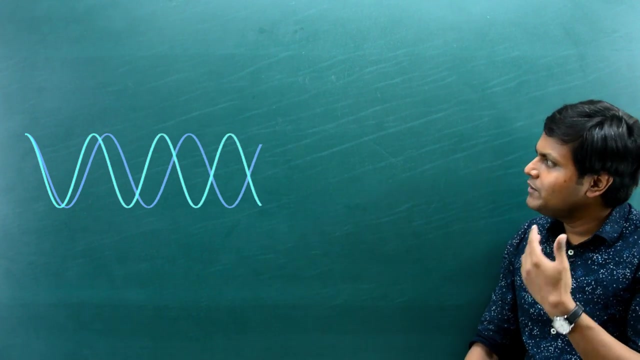 let's suppose the interesting, the peculiar thing about this is that both these two waveforms have different frequencies. so when, let's suppose a particular neutrino is emitted in some kind of a particle interaction, both these two waveforms propagate through space. but they propagate in such a manner: because of the slight difference in the frequency they go in and out of phase. 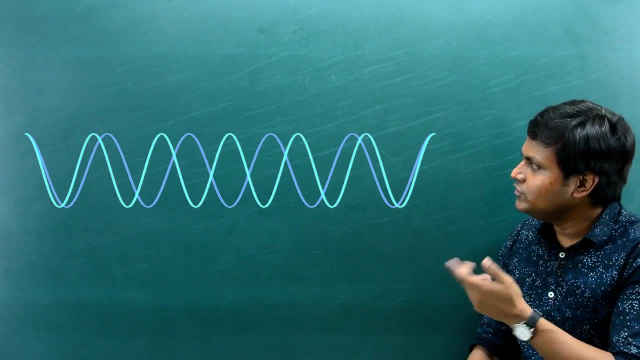 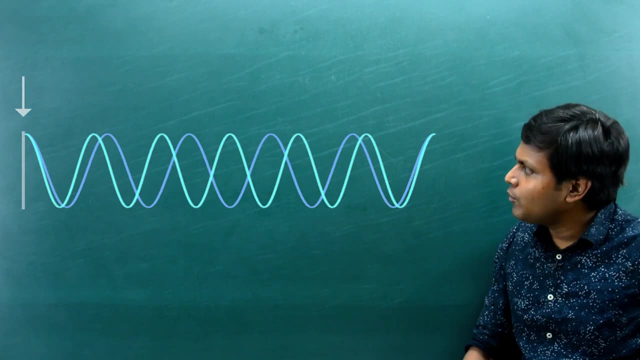 with respect to each other. so if they were emitted such that both these two waves were completely in the moment, the particle interaction happened. but with time, as the particle propagates, they go out of phase and they reach a point where they are completely out of phase, 180 degree out of phase. 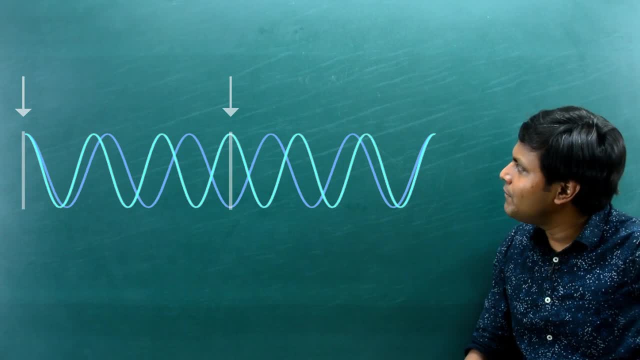 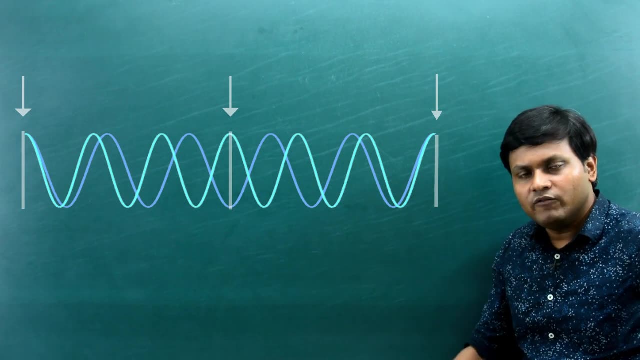 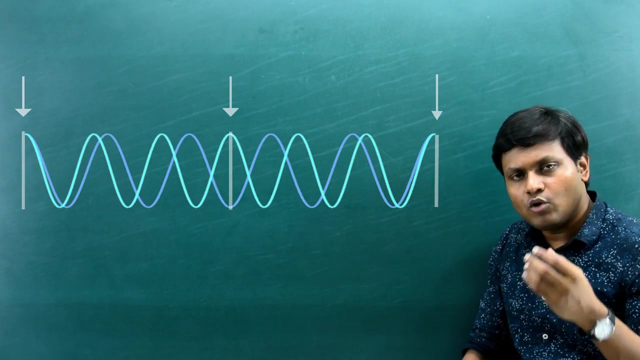 with respect to each other, and then again, after some time, they come back and are in phase with respect to each other. this kind of a thing keeps on happening periodically over time. so now what we can do is we can define the flavor of the neutrino, which is the electron neutrino or the muon neutrino. 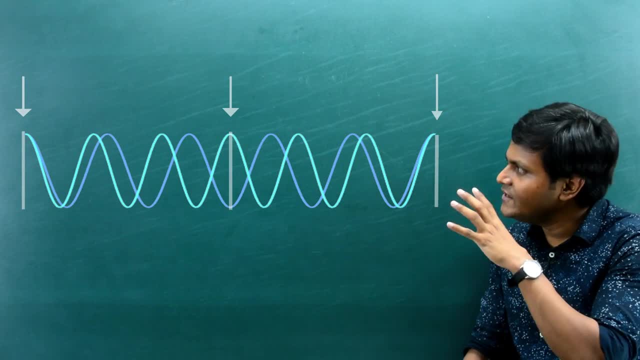 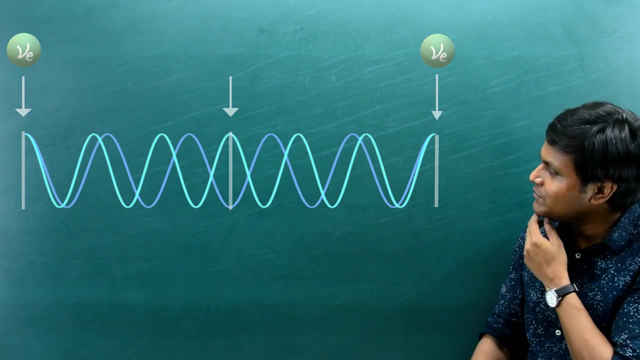 so we can define the flavor of the neutrino by. let's suppose the electron neutrino is nothing but when both these two waveforms are completely in phase with respect to each other, while the muon neutrino is nothing but when both these two waveforms are out of phase with respect to each. 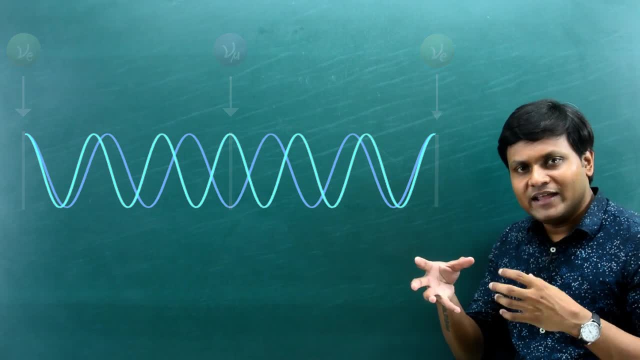 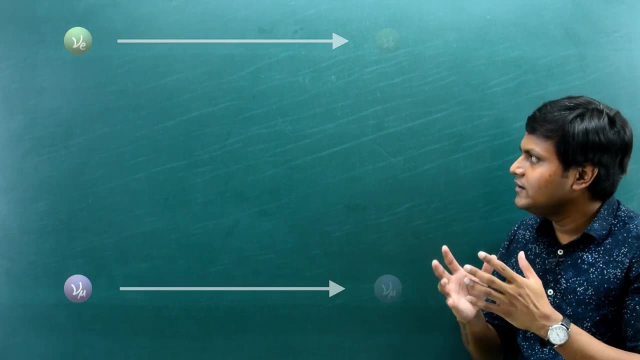 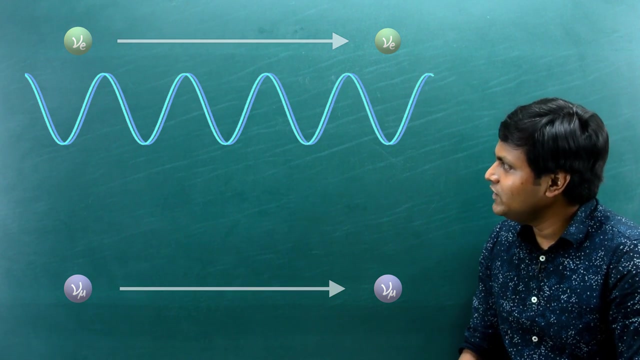 other. so, in a sense, if the electron neutrino and the muon neutrino have their identities intact as they propagated through space, we can, in that particular case, visualize that both these two waveforms will be in phase for the case of the electron neutrino, while for the case of the muon. 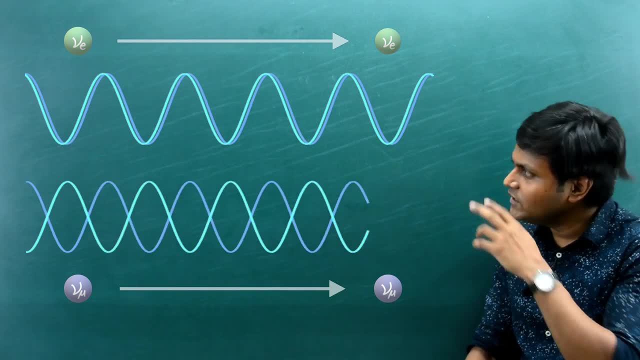 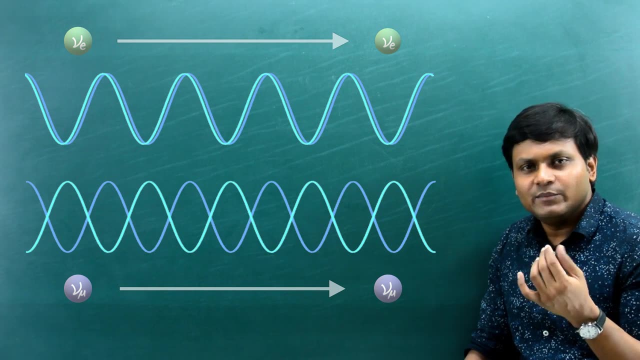 neutrino. both these two waveforms will be completely out of phase, but in both these two cases interesting thing is that the frequencies are same. however, in reality it's a little bit more complicated in the sense that the frequencies of these two waveforms are not necessarily same. so 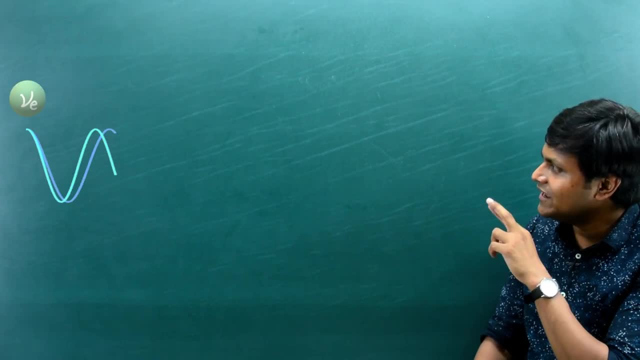 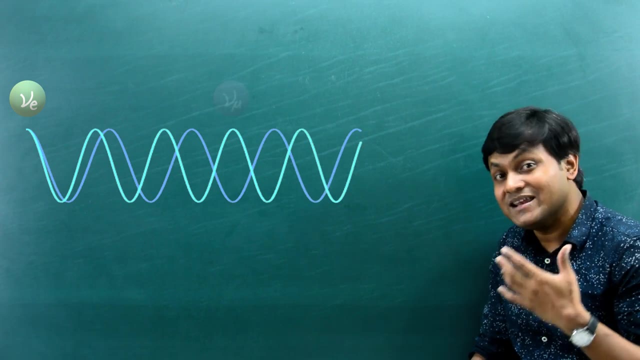 when an electron neutrino is emitted in an interaction, these waveforms are in phase, but with time, as the neutrino propagates, they go out of phase. so these are actually out of phase of phase, and they reach a point where they're completely out of phase. so which represents, let's 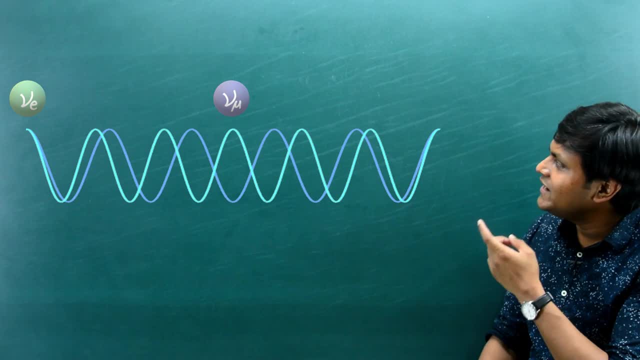 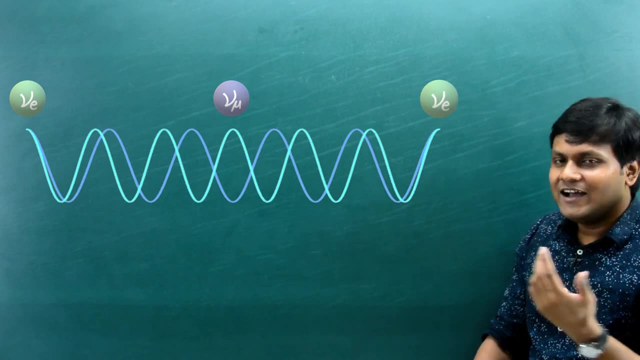 suppose, as we are defining it, a muon neutrino, which then again reaches a point where the waveforms are completely in phase, which represents an electron neutrino, which then again goes forward and becomes a muon neutrino, and on and on, and on. So, in a sense, what was originally an electron, 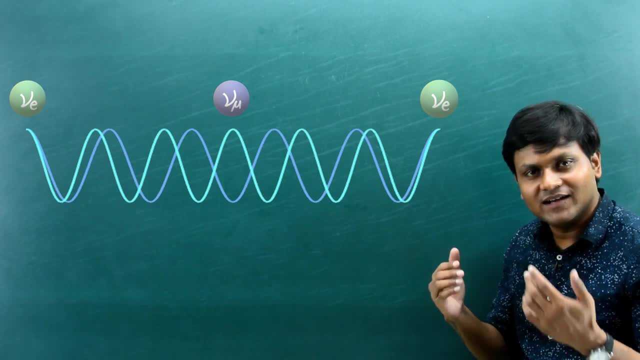 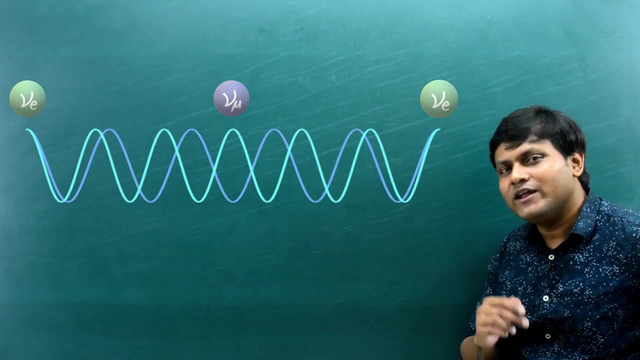 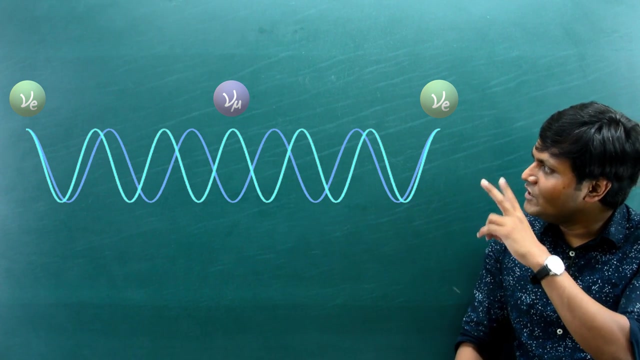 neutrino became a muon neutrino after propagating a certain distance, and then that again became an electron neutrino after propagating a certain distance, and on and on and on. This is the essence of the idea of neutrino oscillations. Now you may ask a question: what about the region in the middle? 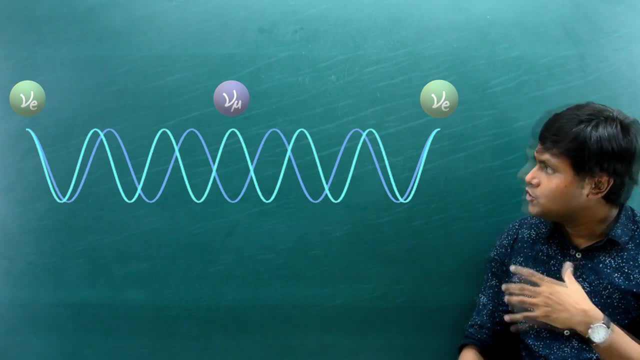 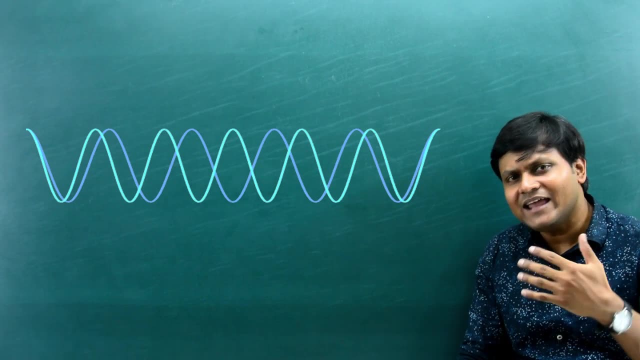 what happens there? Well, because we are dealing with quantum mechanics, so we are essentially dealing with probabilities. So there is a certain probability in the region in between for an electron neutrino to exist and a muon neutrino to exist. So, as you can see here, the probability of 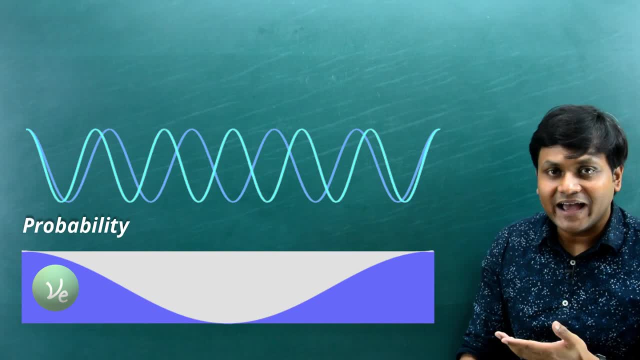 the neutrino being an electron neutrino initially was the higher probability of a muon neutrino to exist and a muon neutrino to exist. So, as you can see here, the probability of the neutrino being an electron neutrino is the highest. but as the 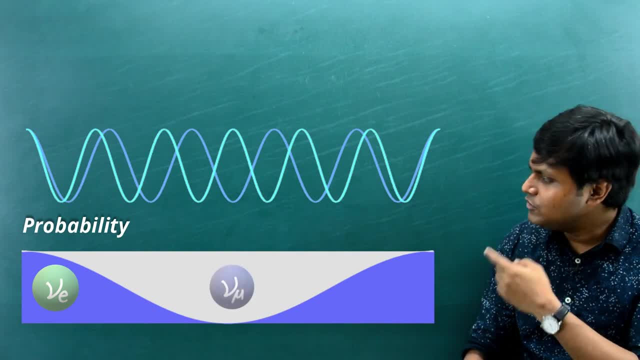 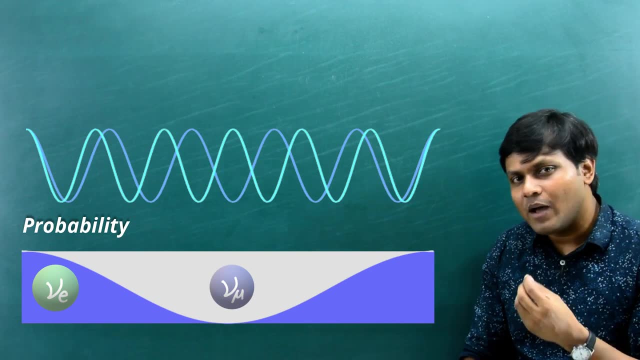 neutrino propagated. it decreased while the probability of being a muon neutrino increased. At a certain point the probability of finding a muon neutrino is maximum, but then again it started decreasing as a probability of finding an electron neutrino started increasing. This kind of 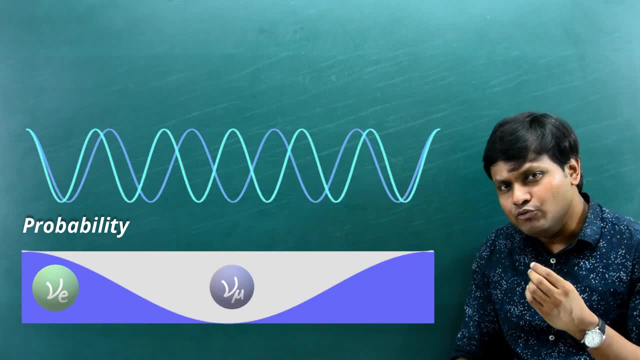 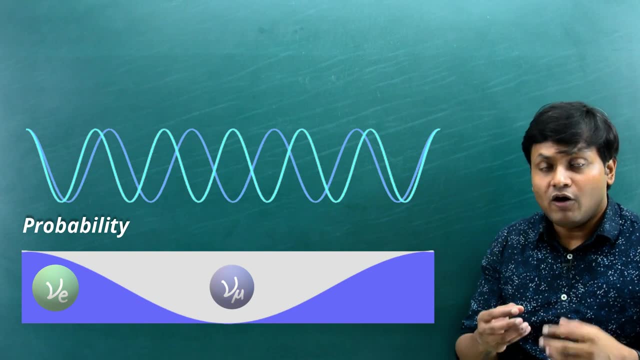 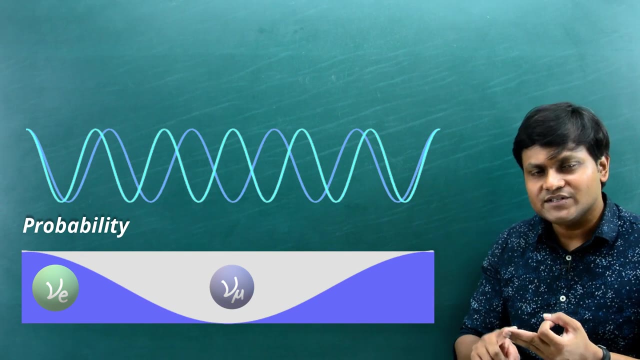 a probability wave of the flavor of a neutrino keeps on oscillating over and over again as the propagates to space. This is the idea of neutrino oscillation: The probability of whether or not the neutrino is in any one of the flavors the electron or muon family is oscillating. 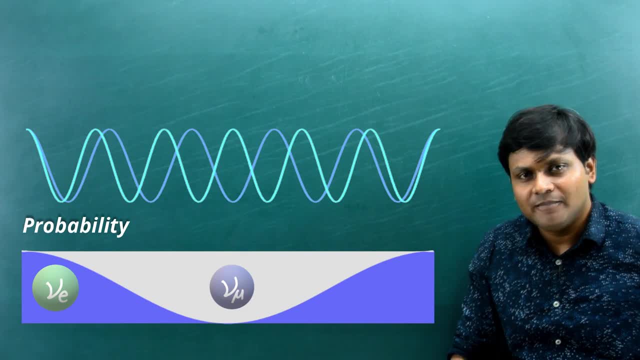 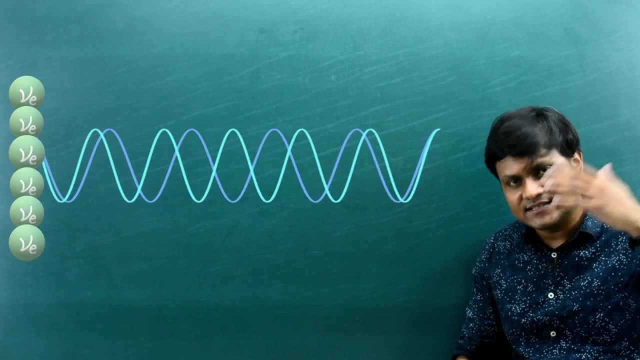 periodically as the neutrino goes from point A to point B. Now what is the idea behind probability? It simply means that let's suppose there are a bunch of electron neutrinos which were created initially at the sun. let's suppose then after some time they will become a mixture of electron and 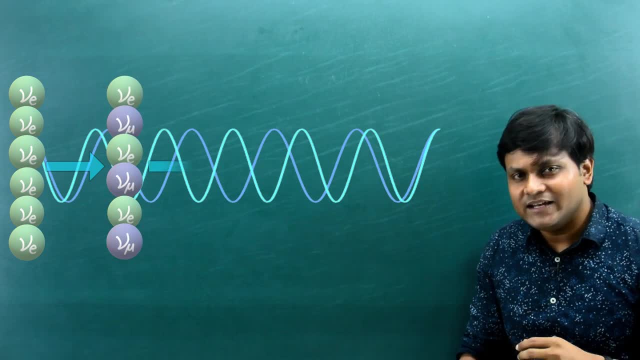 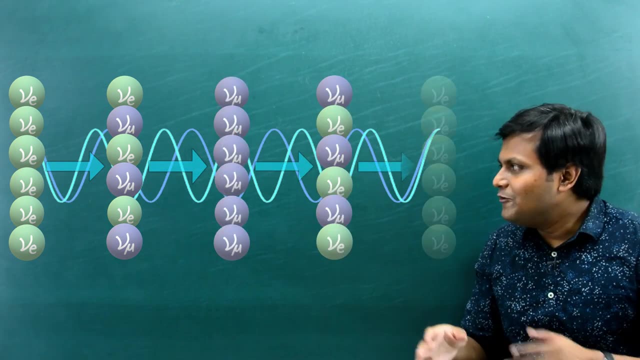 muon neutrinos, while after some time most of them will be dominated by muon neutrinos which again after some time, will become a mixture of electron and muon neutrinos. So this is the idea of probability. So I hope that makes a little bit of a sense to you as to what the neutrino oscillation means. 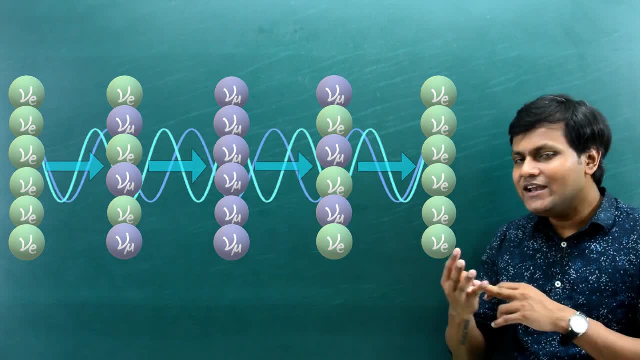 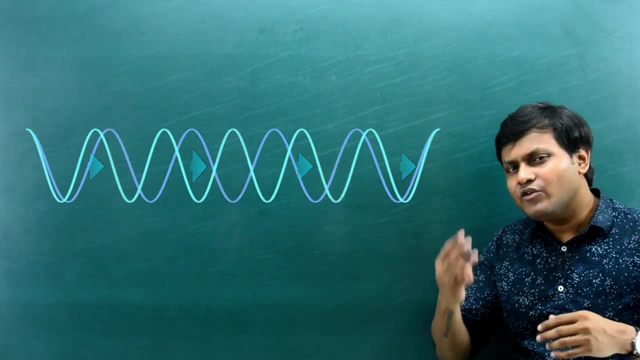 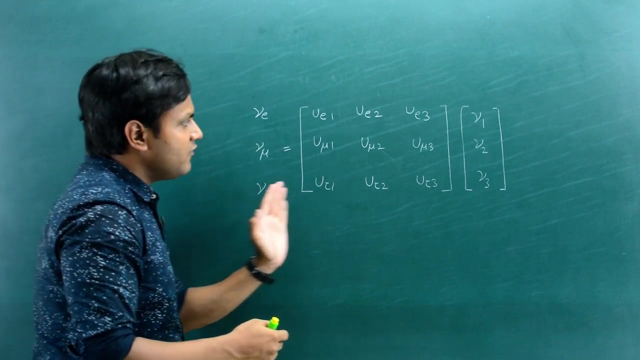 Now I told you that there are three distinct flavors right, and three distinct mass eigenstates. so in that same way we can also visualize the sort of a mixing of these three different states. So the three flavors are the result of a mixing of these three mass states. 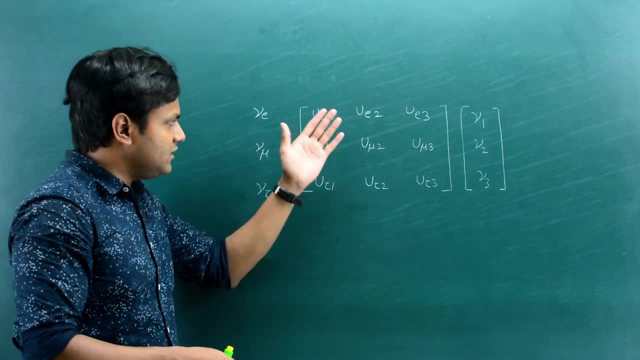 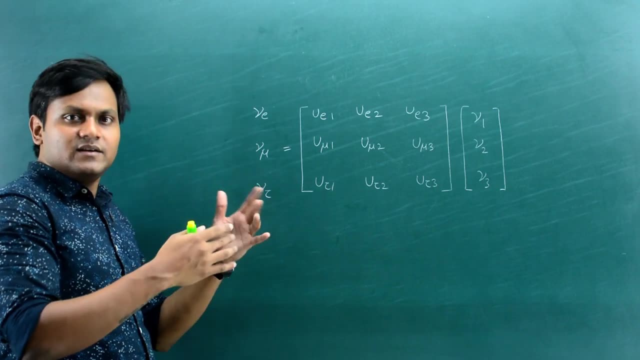 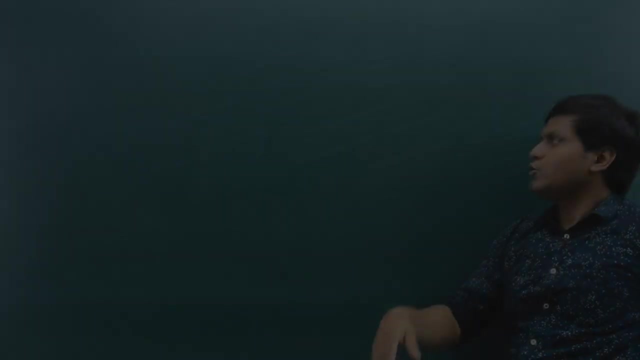 So, again, this is a pretty simple process which involves this kind of a matrix. the terms and the terms associated with the this matrix is not important for our discussion, but we can represent them exactly by using the same kind of a waveform that I used for this previous case. So again, if I 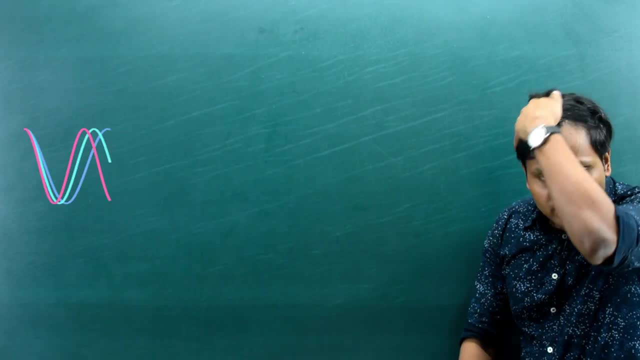 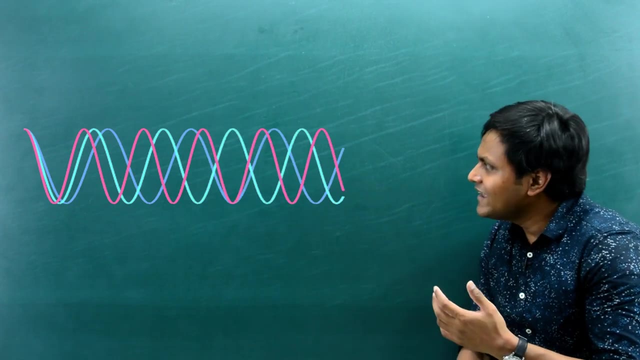 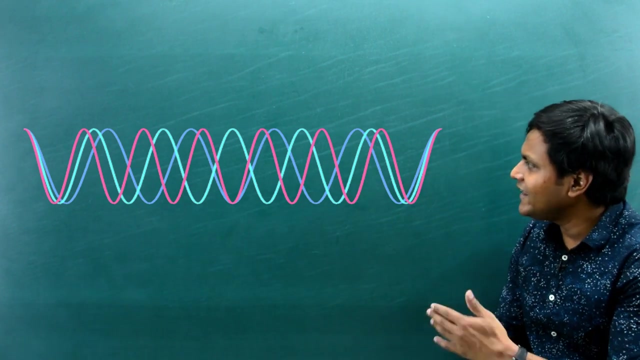 represent the three mass states with sinusoidal waveforms having different frequencies, then you can see that, as the- let's suppose- a neutrino is created, then the matrix is not going to be. you end up getting this kind of a waveform where these distinct waveforms go in and out of phase. 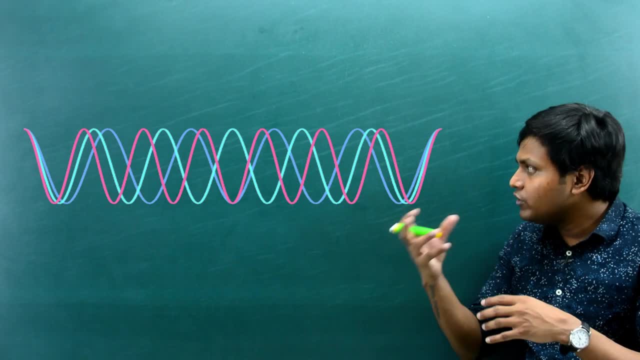 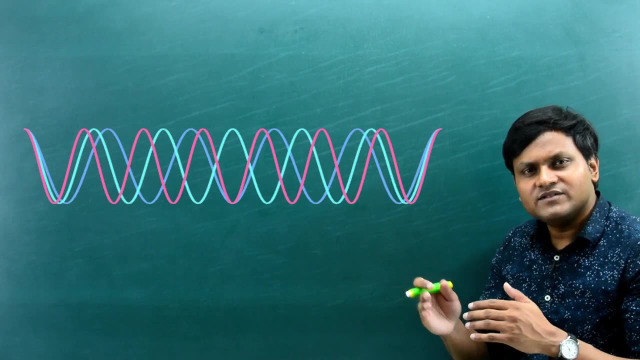 as the neutrino propagates. so we can define the electron neutrino or muon neutrino or the tau neutrino to represent a particular mixing at particular points where the waves are at distinct phases. so let's suppose i represent the electron neutrino as when all 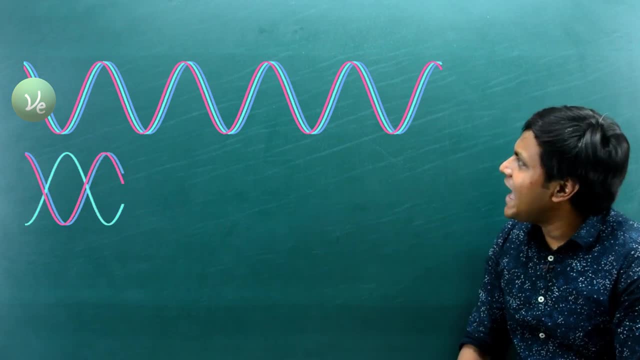 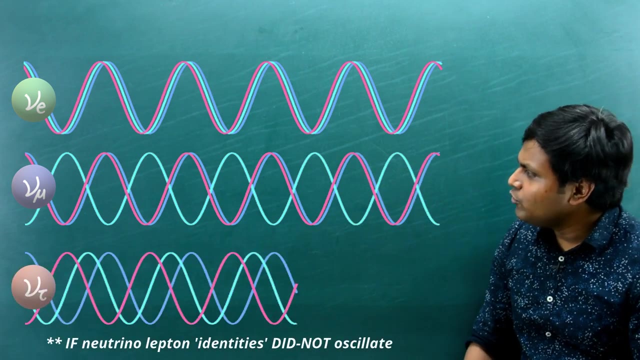 of these waves are in phase with respect to each other and i represent the muon neutrino, as when two of them are in phase, one wave is out of phase and i represent the tau neutrino, with a little bit of more of a complicated form when a neutrino- let's suppose an electron neutrino- is created. 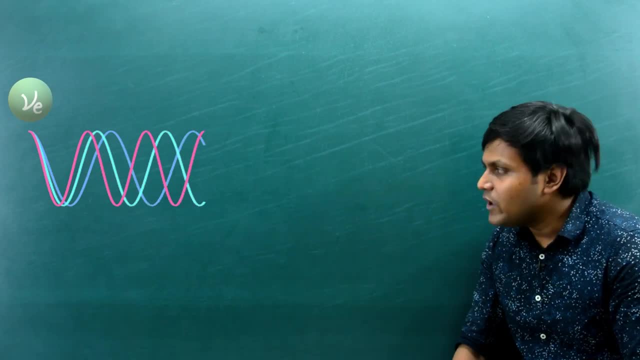 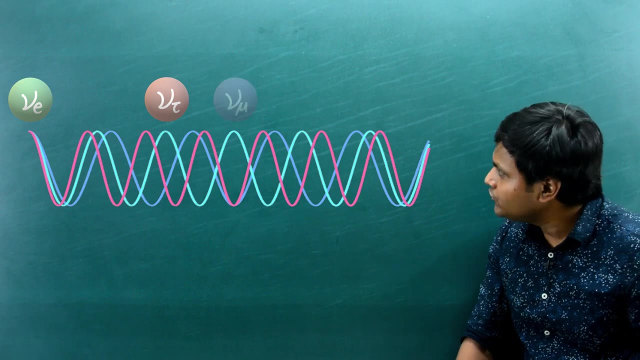 because there is a tiny difference in the frequency of these waveforms. it changes its identity after some time. you end up getting the tau neutrino, then you end up getting the muon neutrino, then you end up getting the tau neutrino, then you end up getting the electron neutrino, and 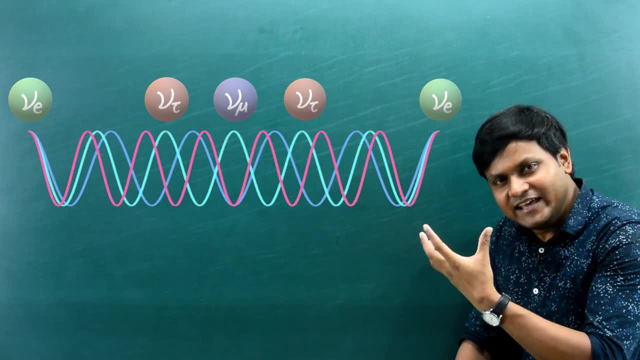 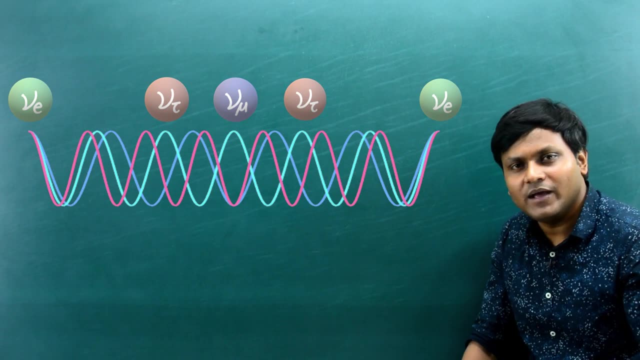 on and on and on. so, as the electron neutrino is created initially, after some time there is a probability that it might remain an electron neutrino, or it might become a muon neutrino, or it might become a tau neutrino. now this whole discussion. i have tried to create this video. 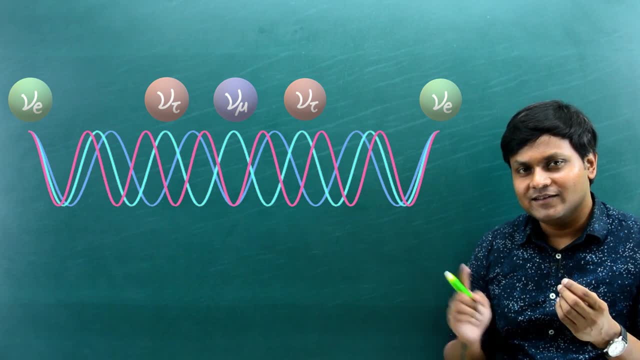 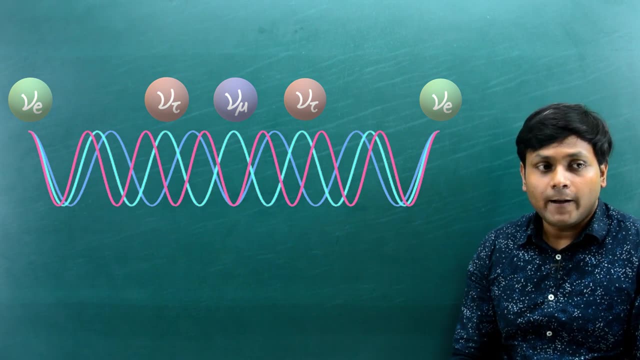 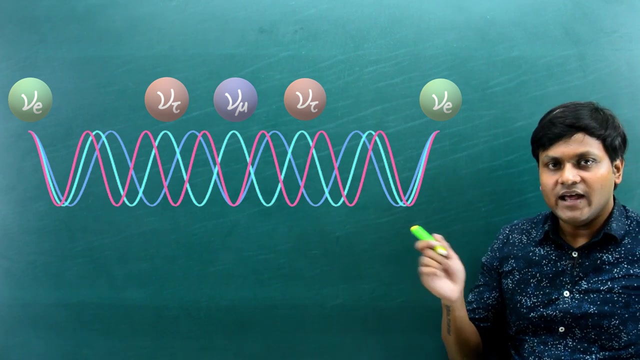 just to give you a little bit of a feel flavor, so to speak. you know neutrino flavor, so i wanted to give you a little bit of a flavor of what it actually means. okay, because, uh, i am using an analogy which is, to be very frank, quite simplistic, because the matrix form i, that i 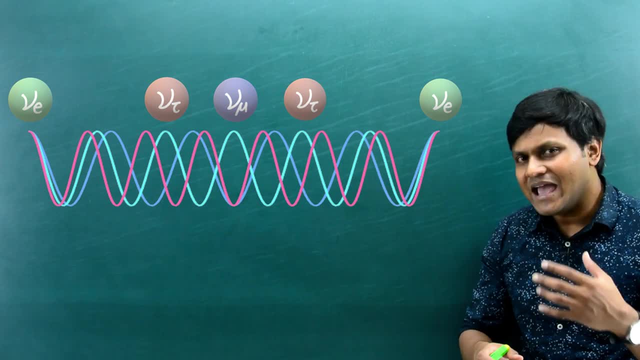 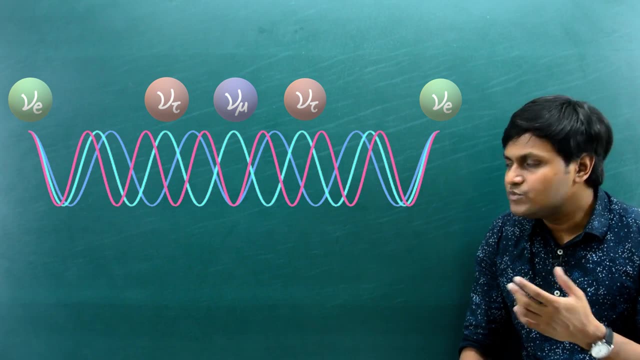 presented to show the mixing of the neutrinos contains imaginary as well as complex terms. so it is not a right to say that the precise manner in which we can represent these quantum states is using these kind of sine waves. but i am only using these sine waves to give you a little. 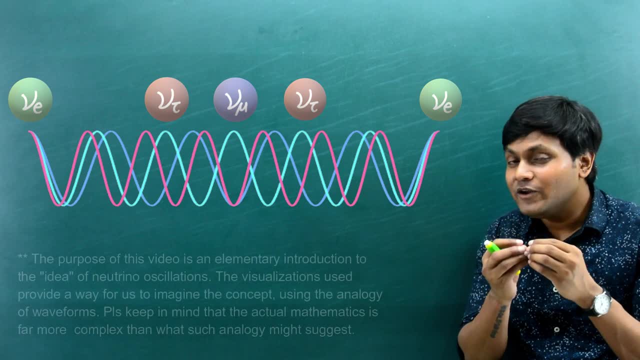 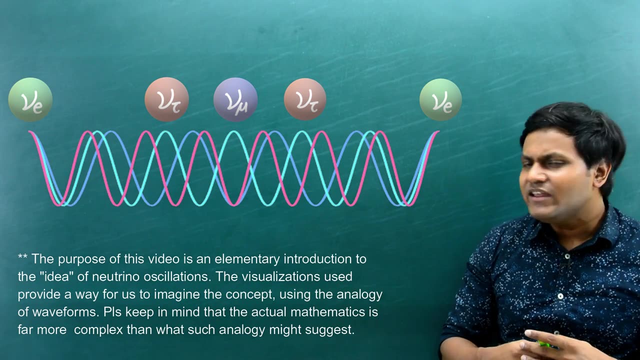 bit of a visualization, a little bit of a taste, a little bit of a flavor of what this idea of neutrino oscillations is. now, of course, this kind of an idea is a very different idea, a very new radical, in fact a very bizarre idea of what neutrino oscillations are, so what neutrino oscillations is now. of course, this kind of an idea is a very different idea, a very new radical, in fact a very bizarre. 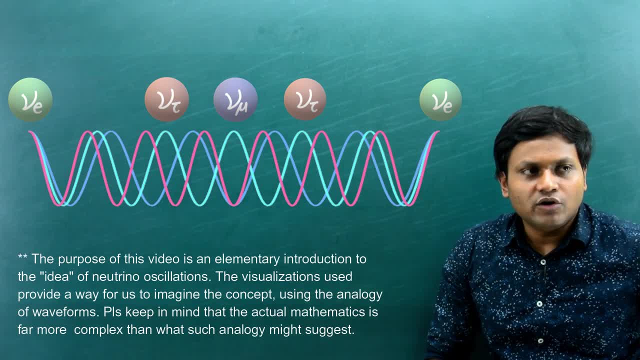 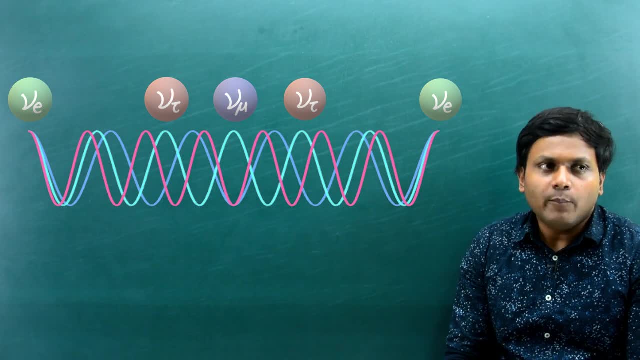 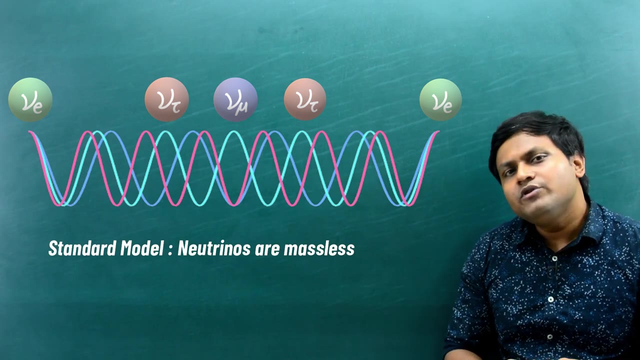 idea, and because of which reason? even though the idea of neutrino oscillations was introduced by quantico orvo in 1960s, it was not accepted as a fact up to the beginning of this particular century. this is because the standard model assumes that neutrinos are massless. so if neutrinos are massless,